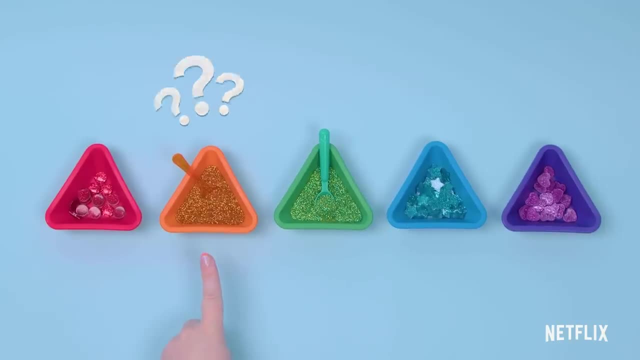 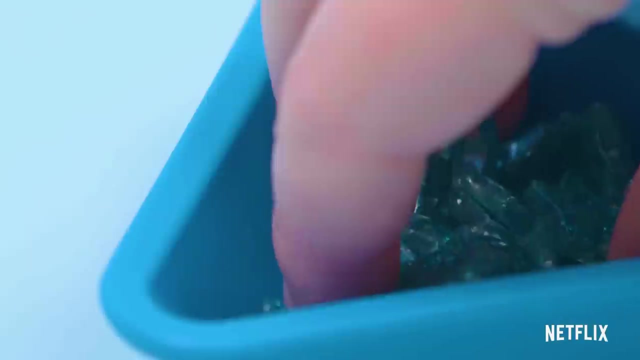 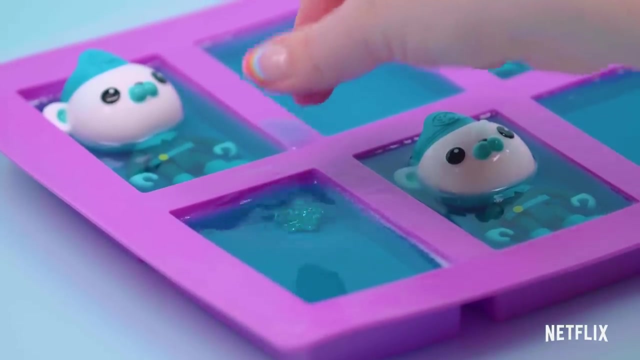 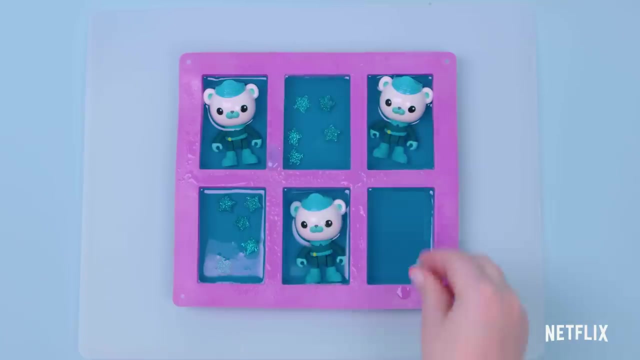 No, that's green, No, that's orange. Is this bowl blue? That's right, this bowl is blue. Aw, cute, Captain Barnacle's is in the soap. Let's make red soap with Professor Inkling. Is this bottle red? 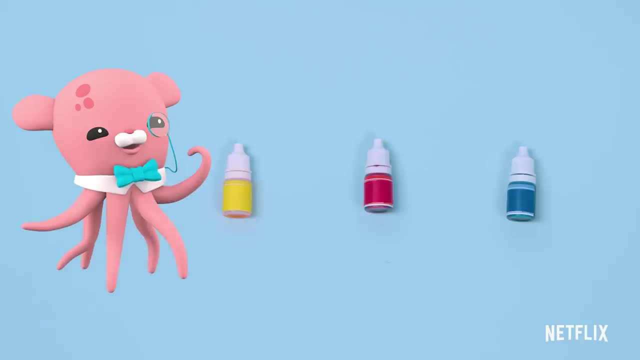 No, that's yellow. Is this bottle red? Yes, you found the red bottle. This is blue. This is orange. This is green. This is black. This is yellow. This is blue. This is green, This is blue. 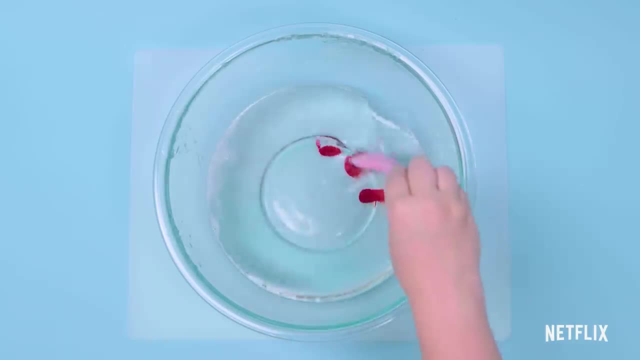 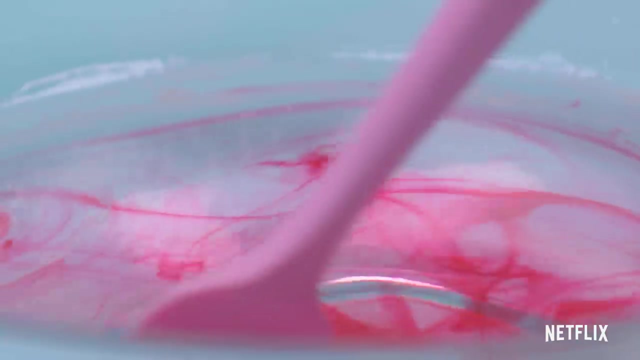 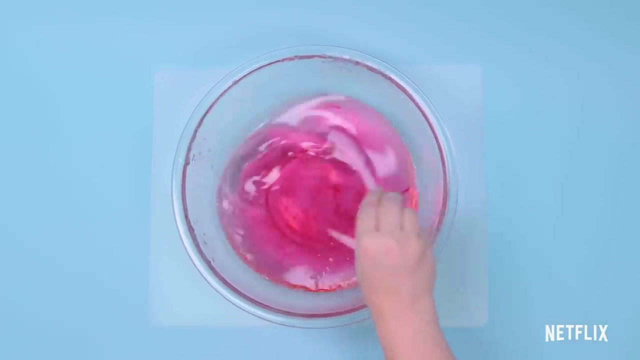 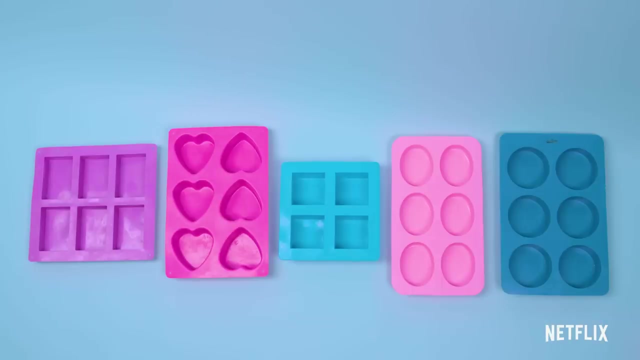 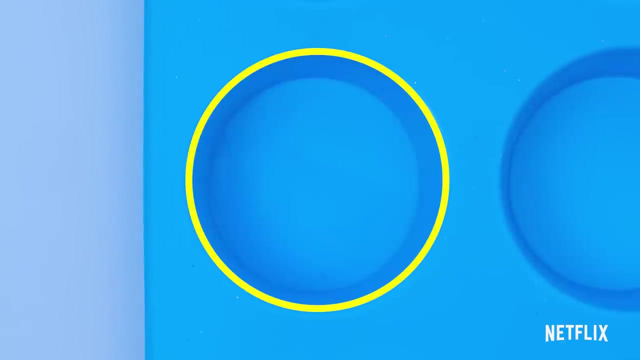 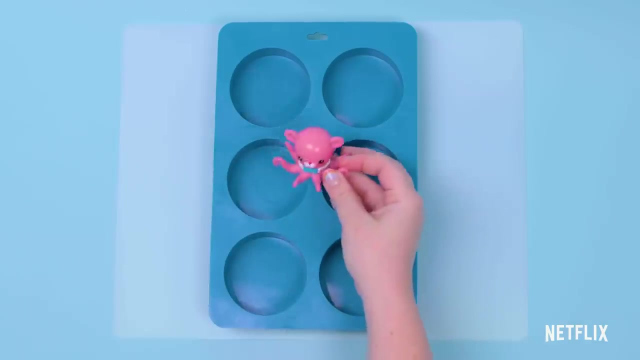 This is blue. This is blue. There is a lot of water in the lift. I'll make the soap water. Time to choose a shape for our soap, Which one of these has circles. That's right, Circles are round. The big ones are round. 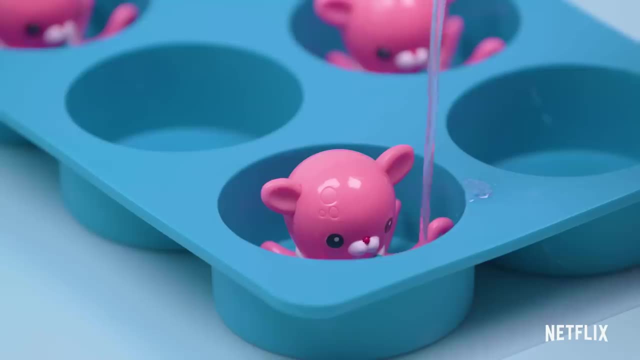 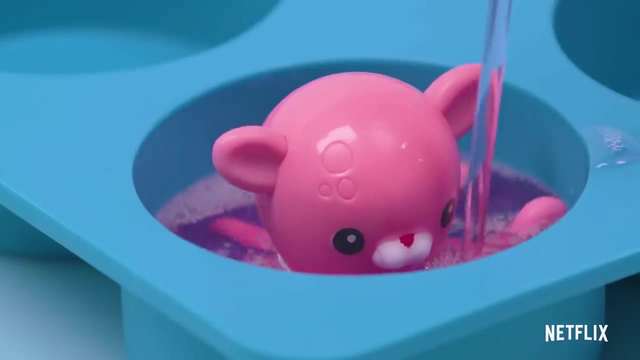 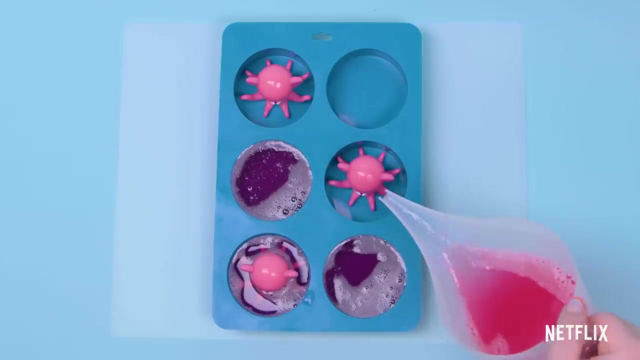 Soap is made of a lot of different materials, such as feel and polymers. Soap is an easy soap to use with a lot of different properties. You can use it to wash your face brush, wash your face with soap and wash your face with soap. 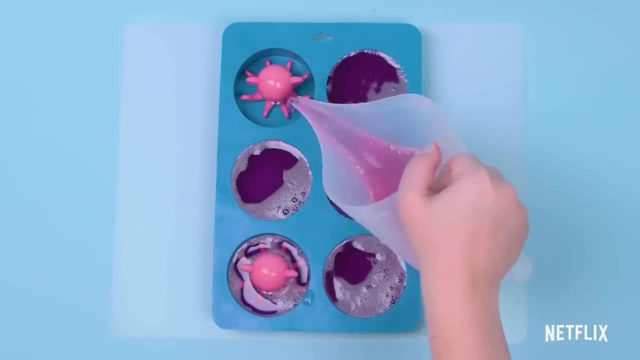 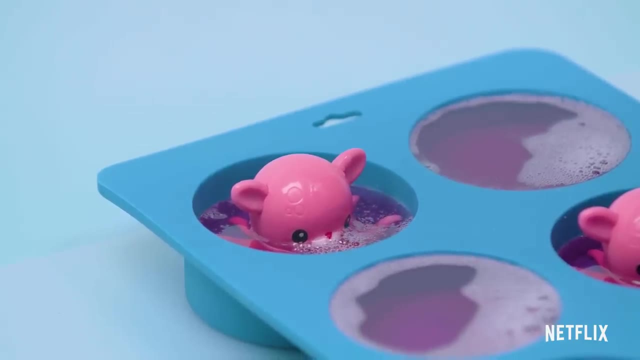 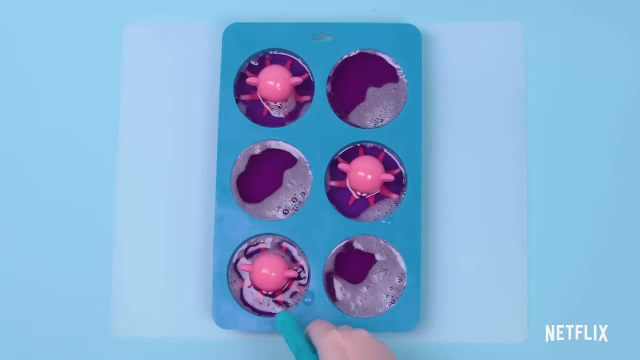 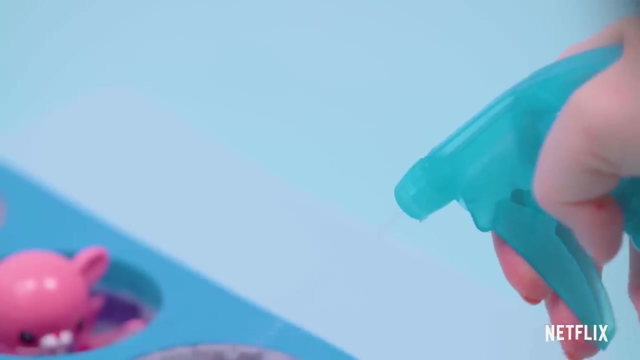 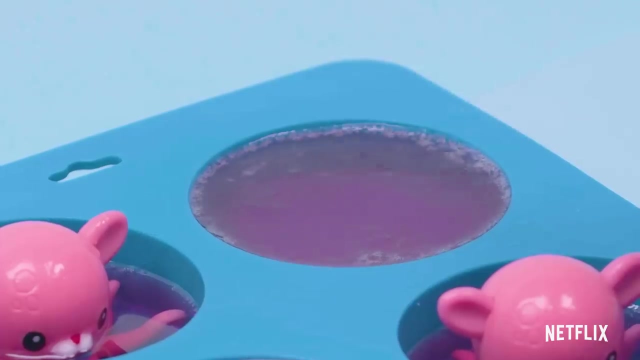 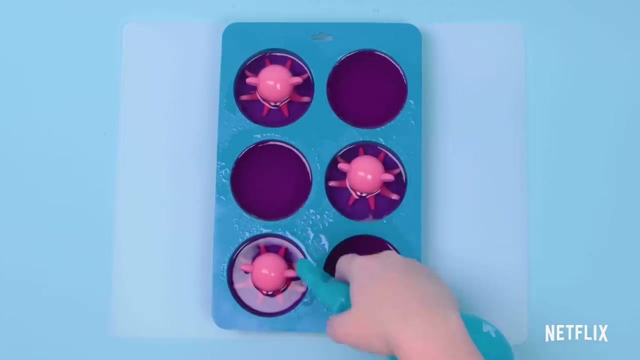 Soap is the softest soap. You can also use it to wash your face with soap. Soap is the softest soap. Soap is a soft soap. Soap is a soft soap. He looks cool in the soap. Let's add red charms to the soap. 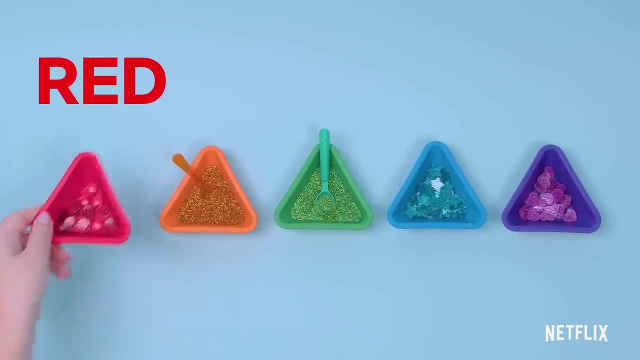 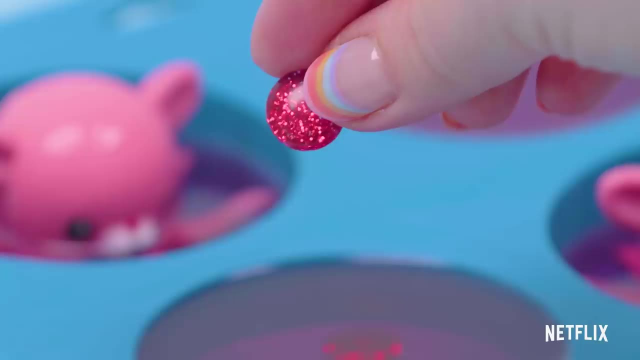 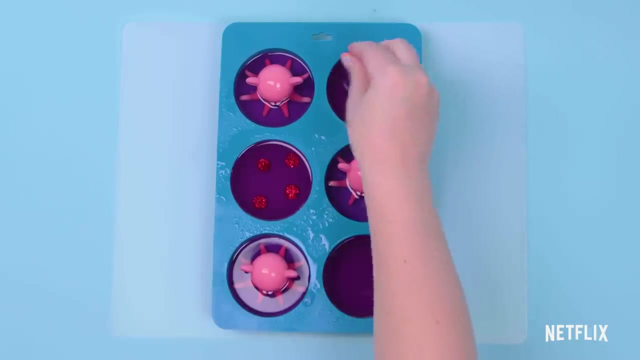 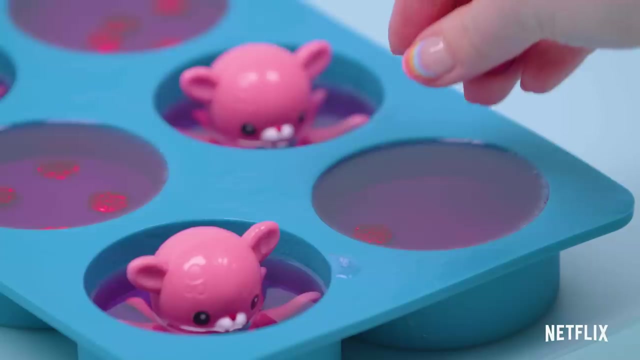 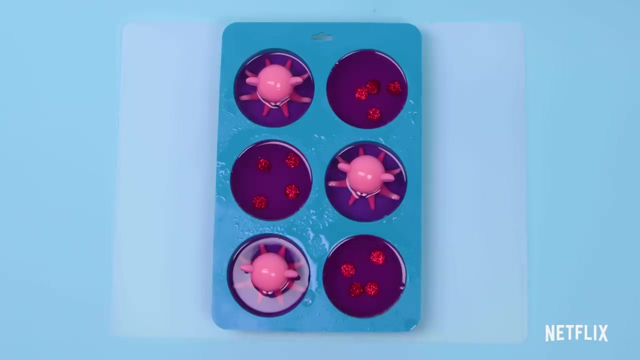 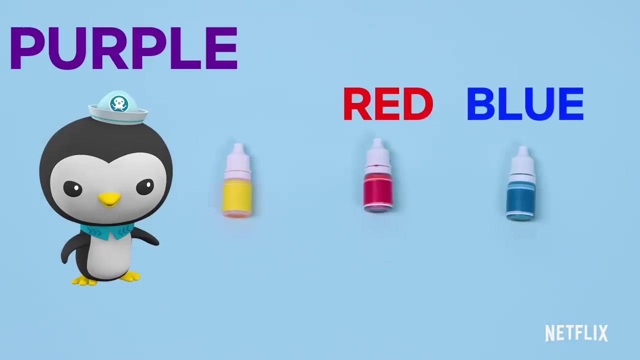 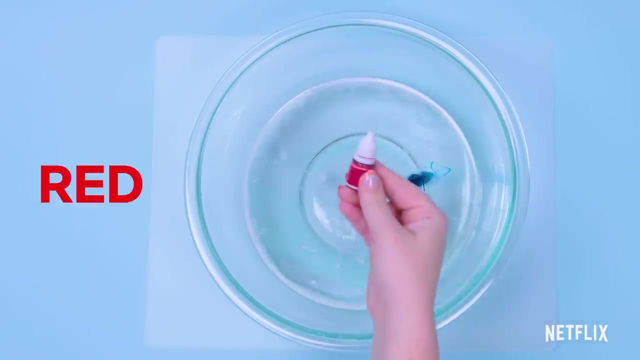 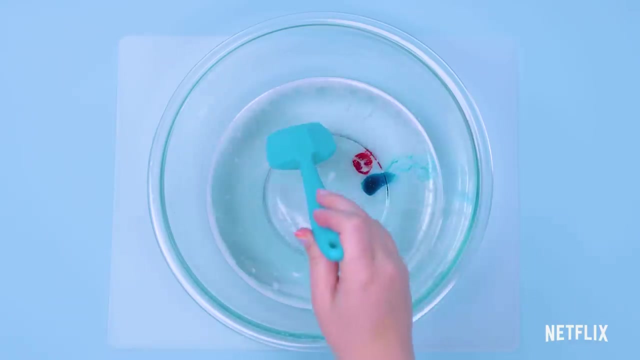 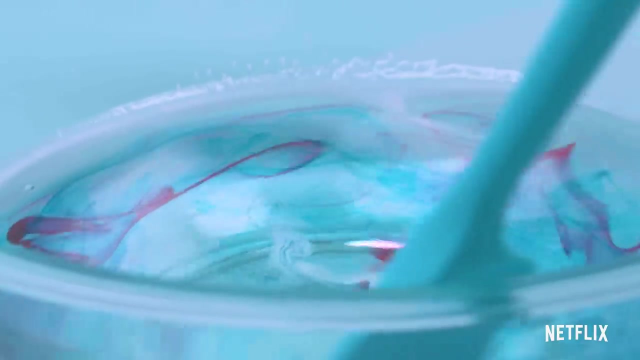 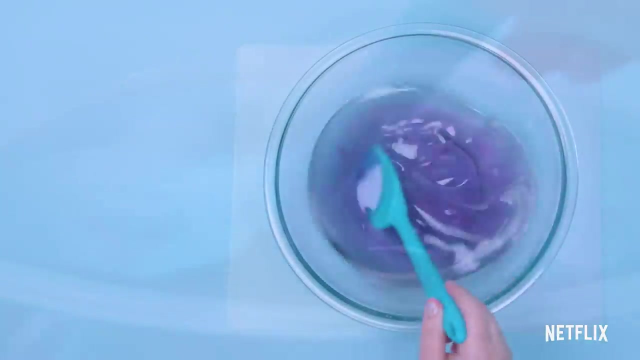 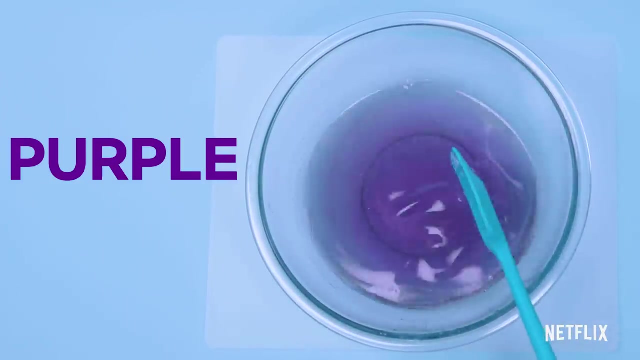 Is this bowl red? Yes, that bowl is red. Okay, Now let's try mixing colors To make purple. mix red and blue. Let's try it: Blue, Red, Yellow. Wow, red and blue make purple. Time to choose a shape for our soap. 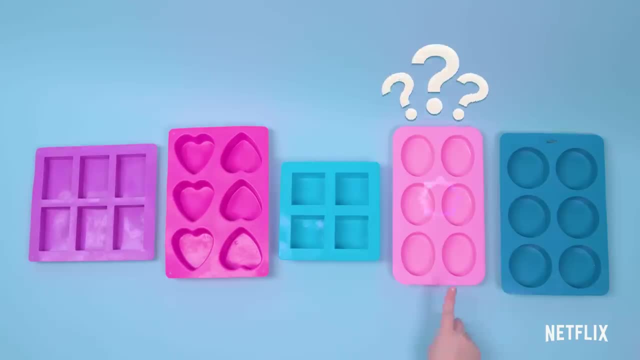 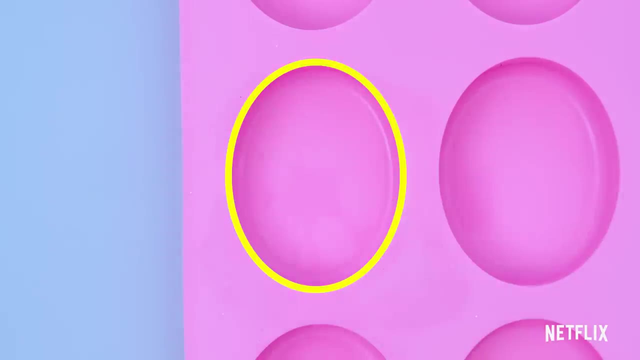 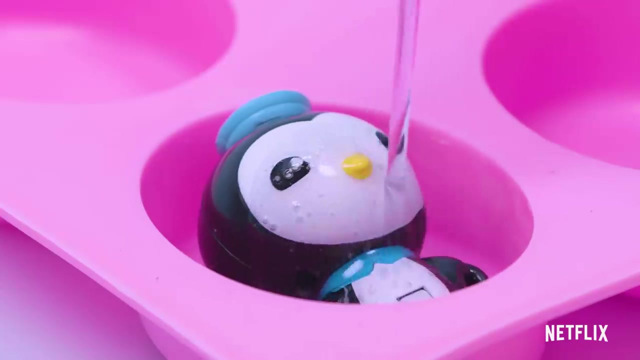 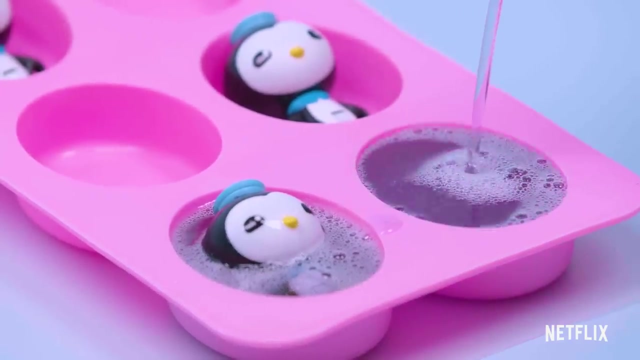 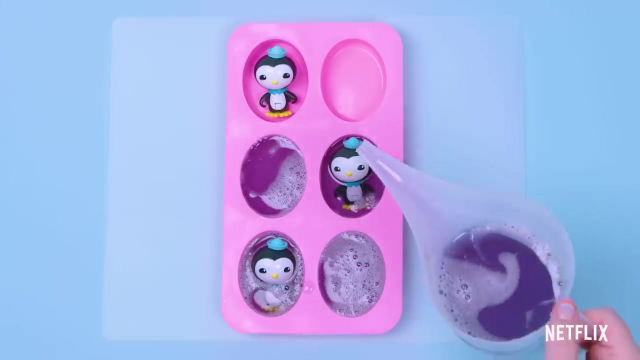 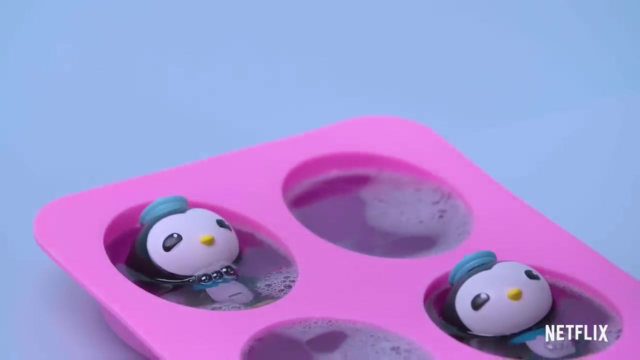 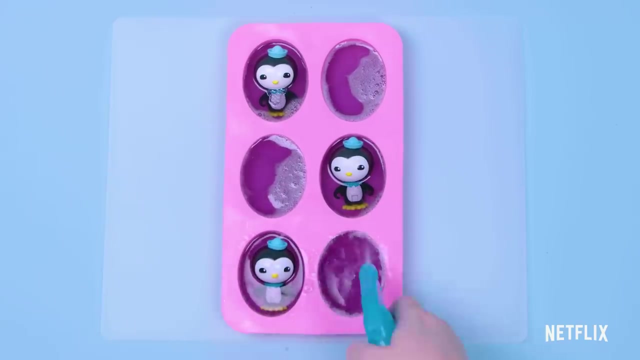 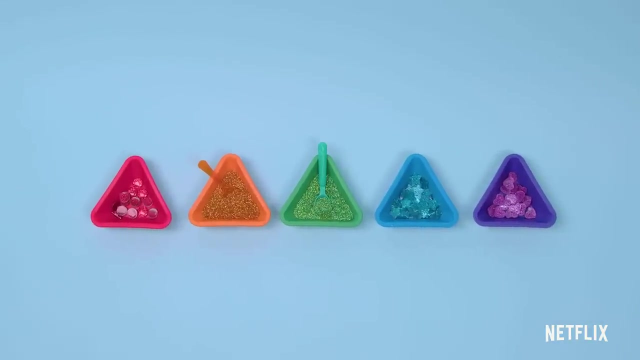 Which one of these has ovals? That's right, it's this one. Let's make soap shaped like ovals. Let's do it. Let's do. it Looks like he's taking a bath in the soap. Let's add purple charms. 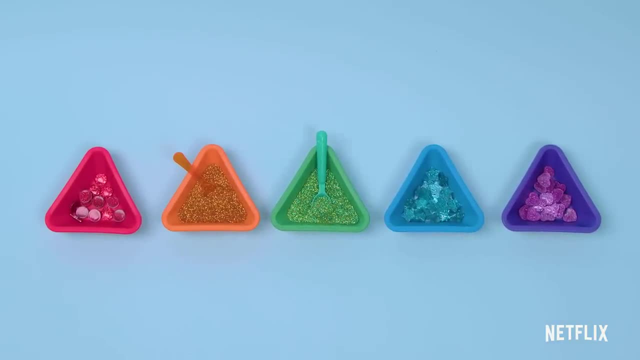 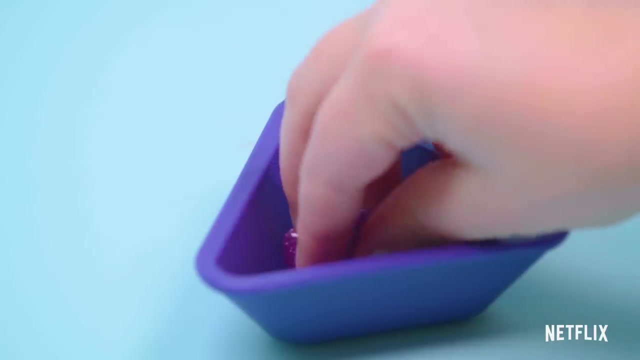 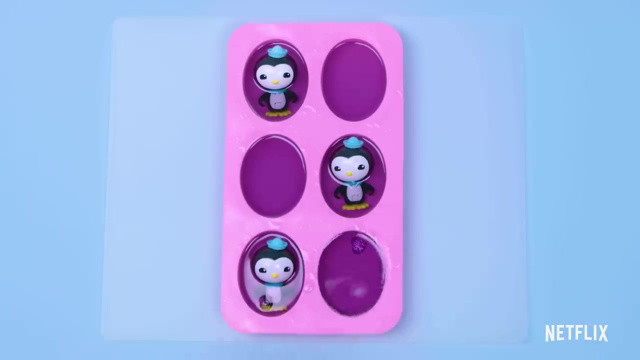 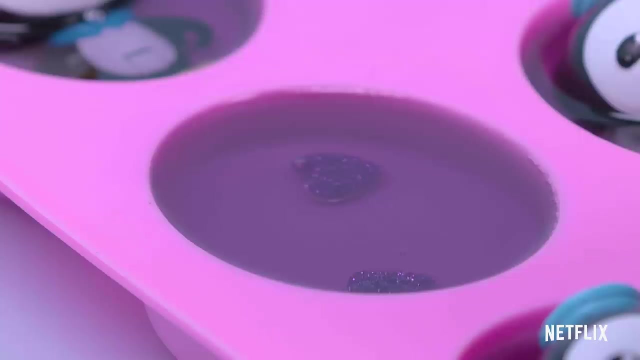 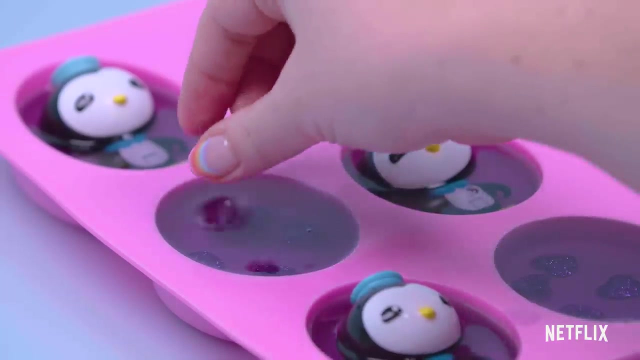 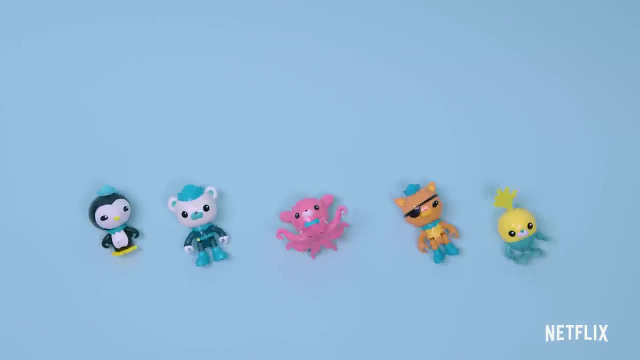 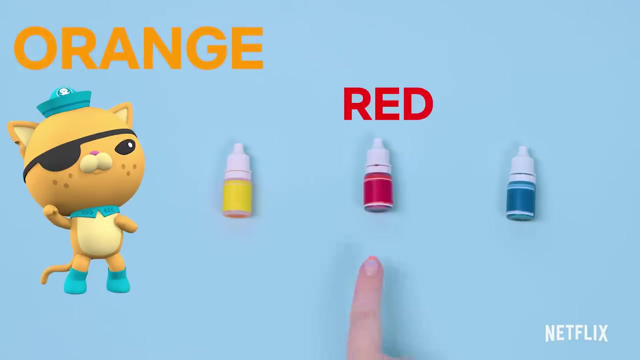 from the purple soap. Let's add purple bowl to the purple soap. Is this bowl purple? Yes, you found the purple bowl. Now let's make orange soap with Quasi To make orange mix red and yellow. Let's try it. 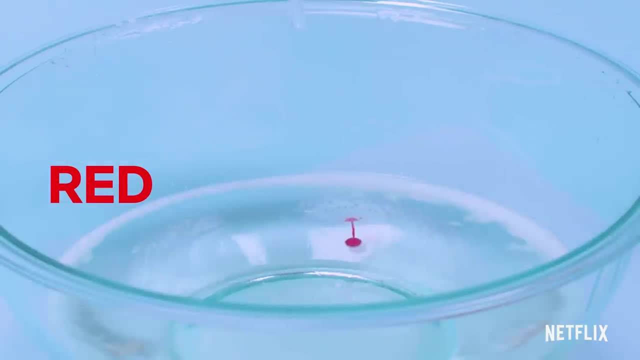 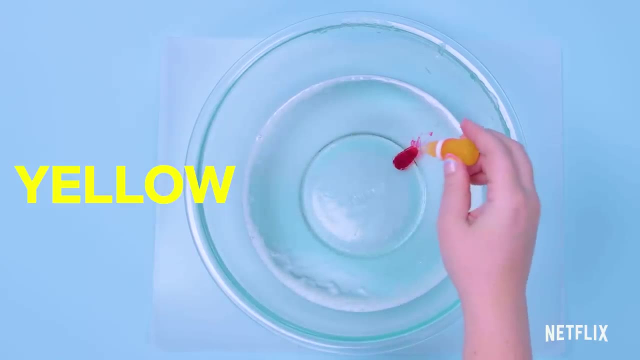 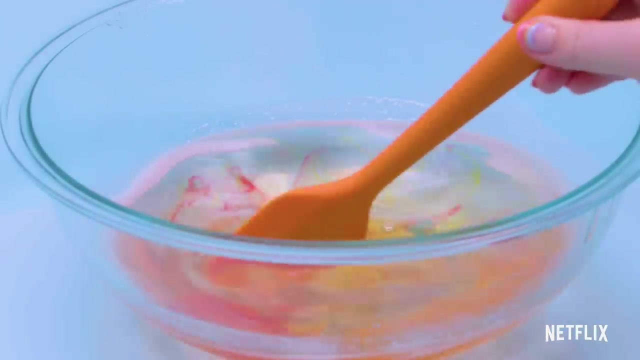 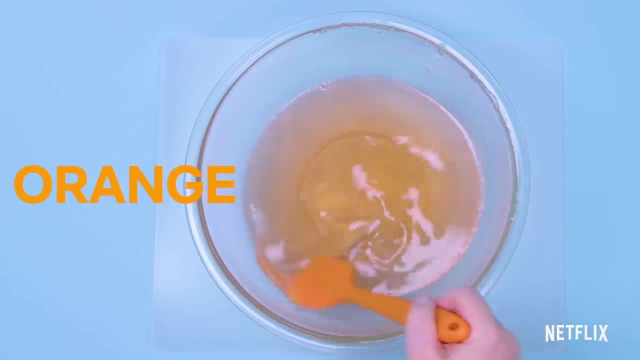 Red Hot sauce, yellow, Try again, Yellow. Wow, Red and yellow make orange Hot sauce. That's so cool. Oh, Hey, Nmondose, I got a friend. Oh, I want to play at the bringer's bowl. 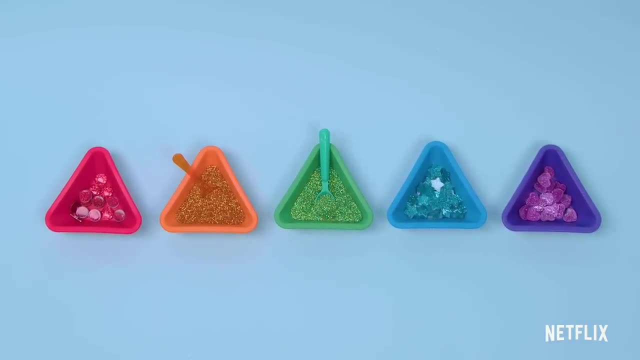 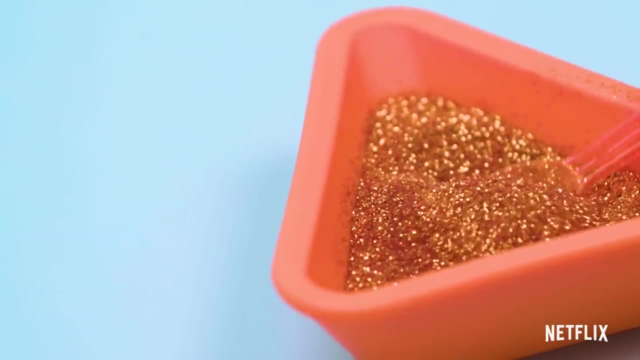 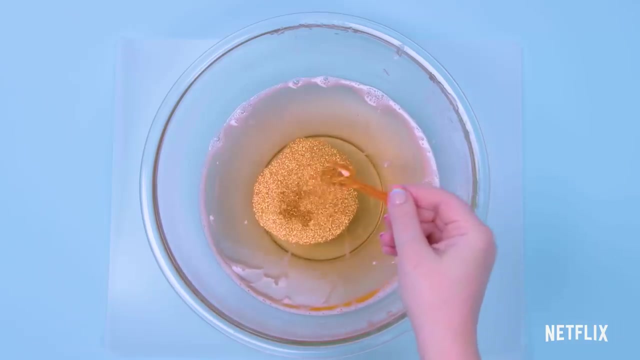 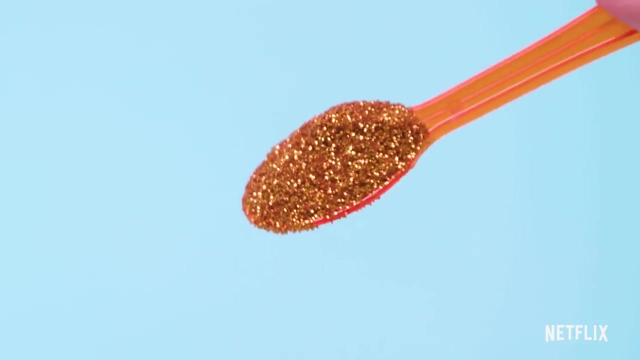 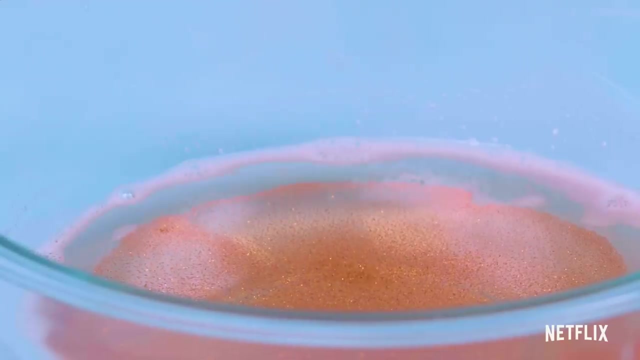 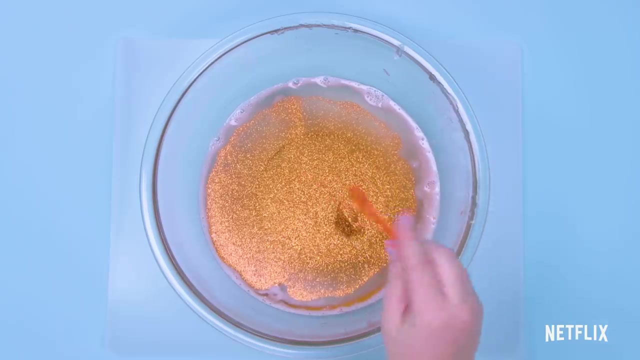 Let's meet Quasi. Let's add orange glitter from the orange bowl. Is this bowl orange? Yes, that's the orange bowl. Let's add orange glitter. Let's add orange glitter to the bowl. Mix it up. Add orange glitter to the bowl. 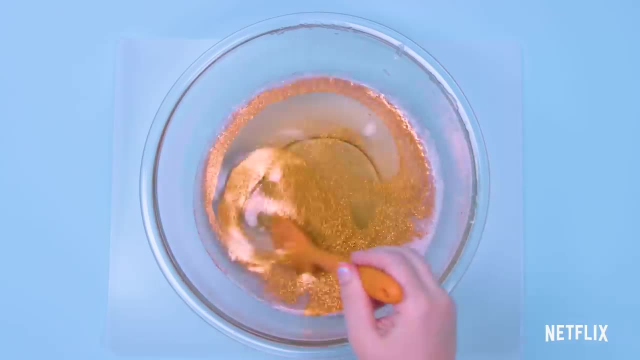 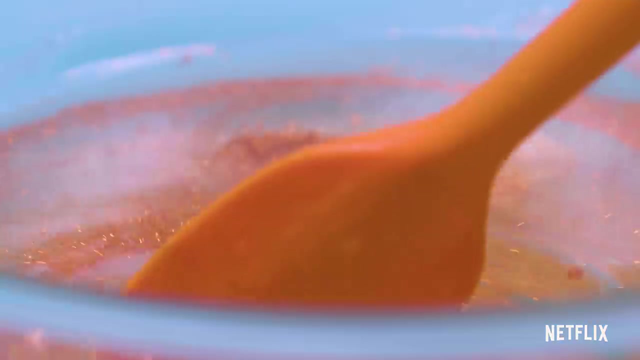 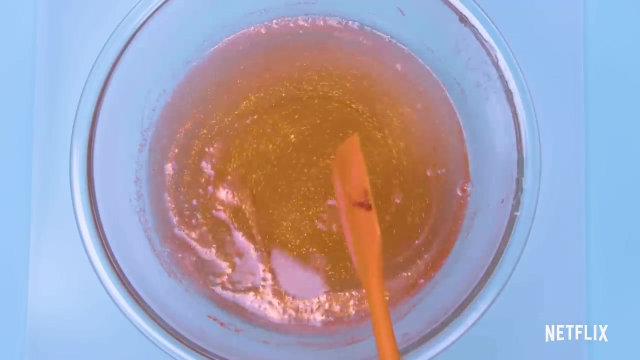 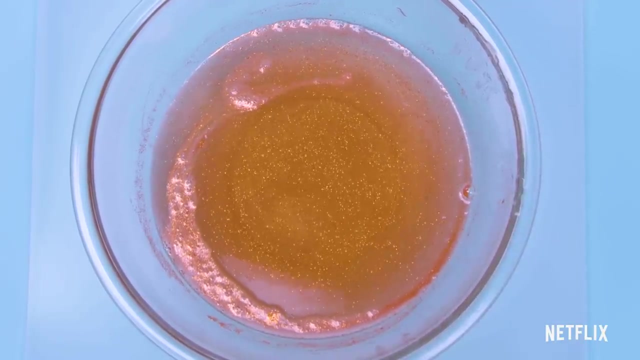 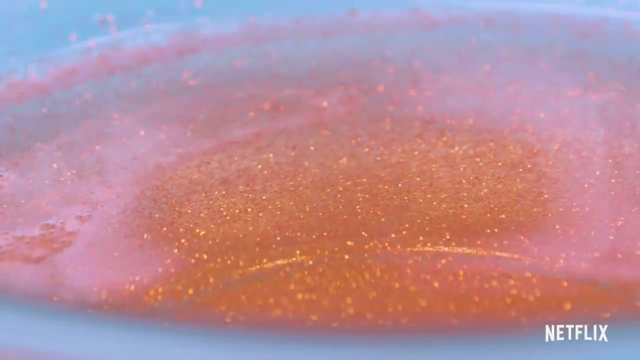 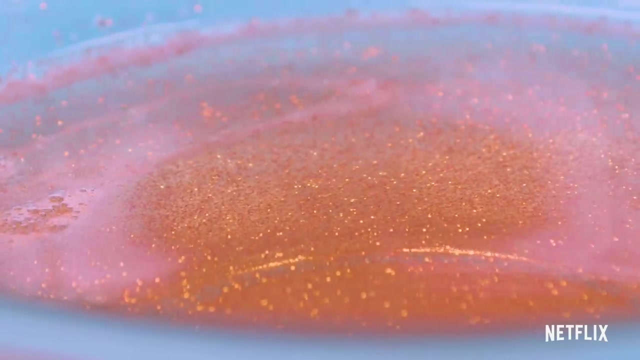 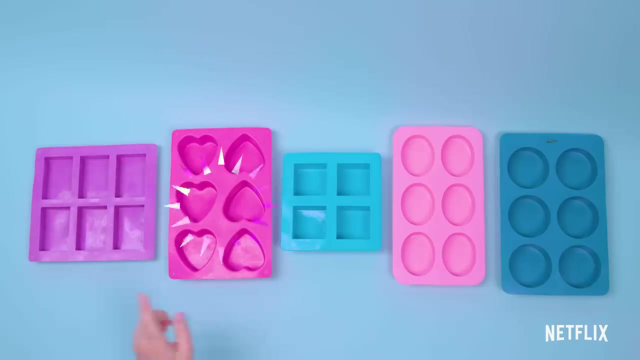 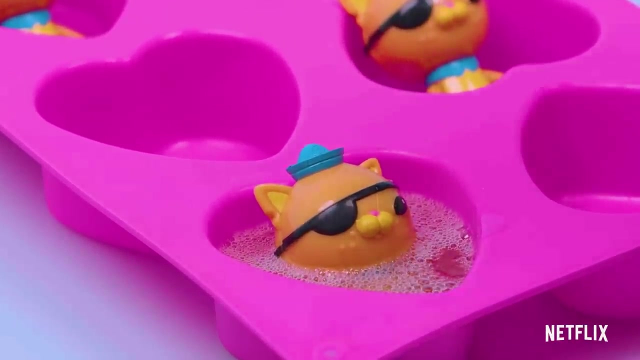 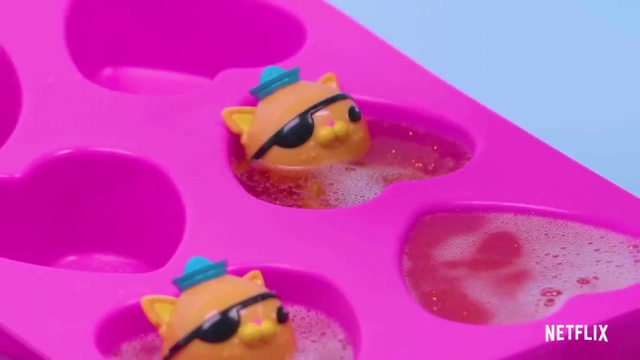 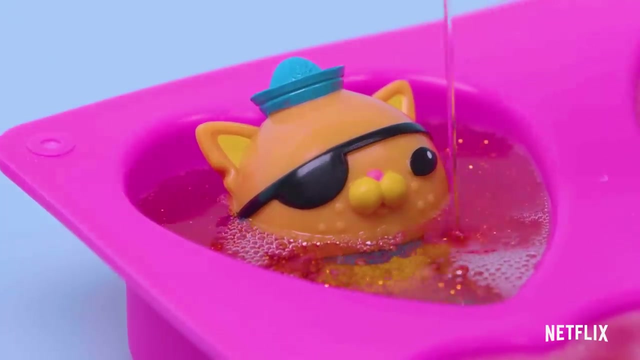 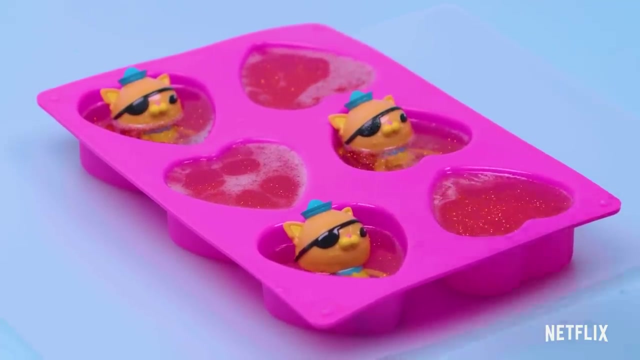 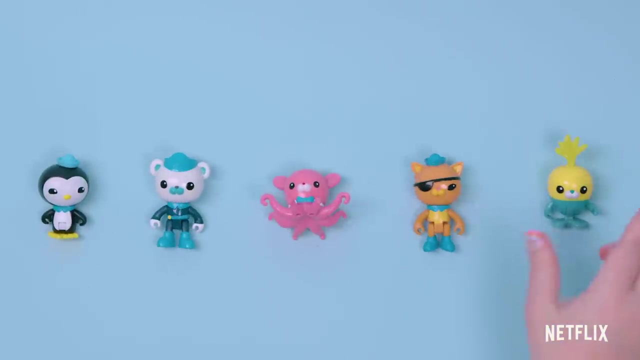 Mix it up. running water. Mix it up. Add orange glitter to the bowl. Add orange glitter to the bowl. Time to choose a shape for our soap. Can you find the one with hearts? That's right, Let's make green soap with TUNIP. 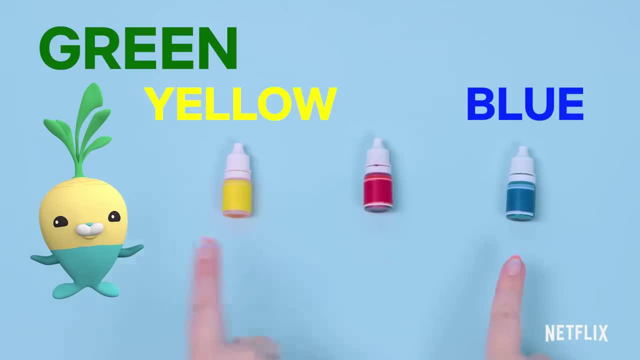 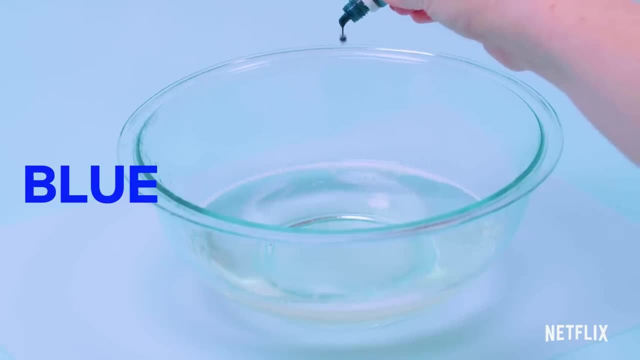 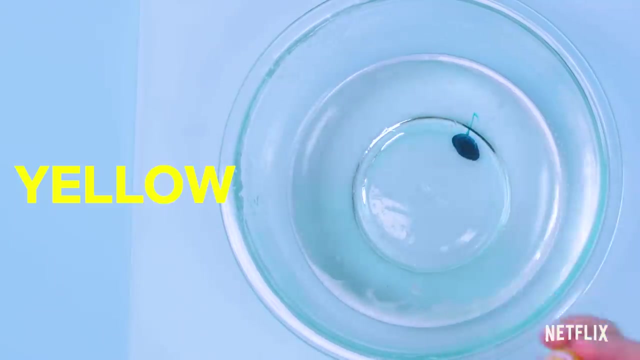 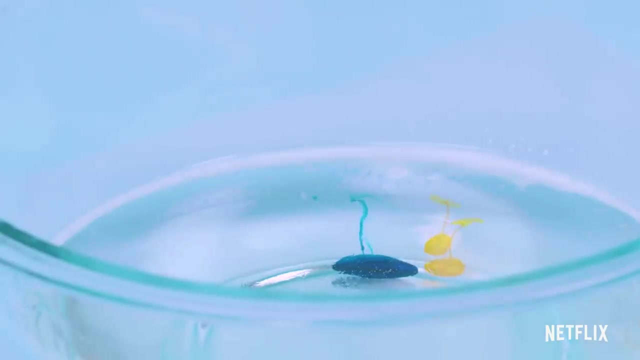 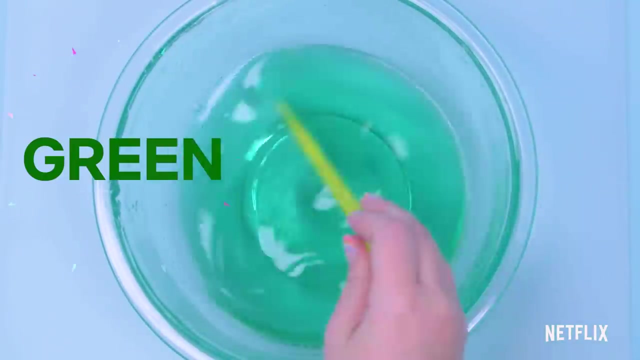 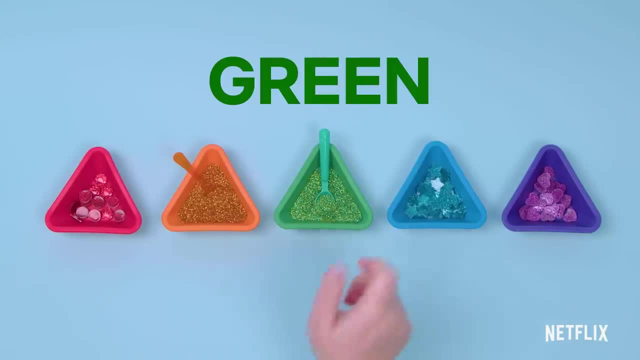 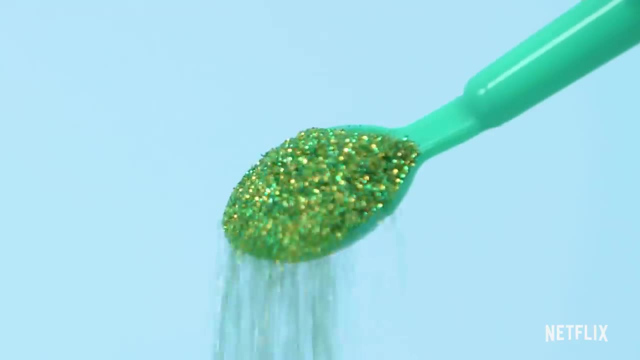 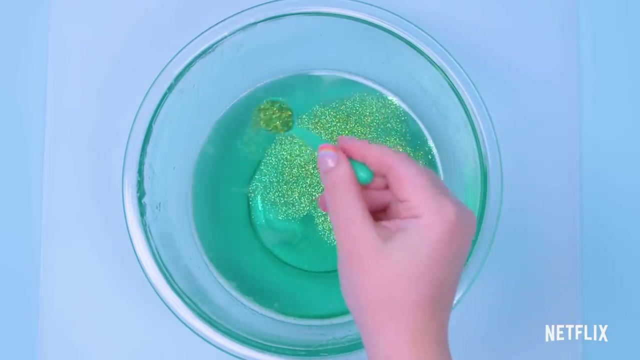 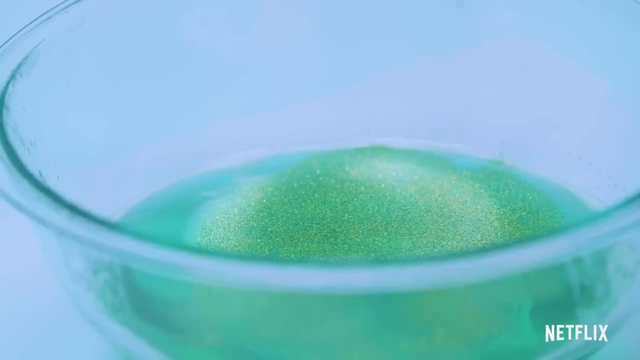 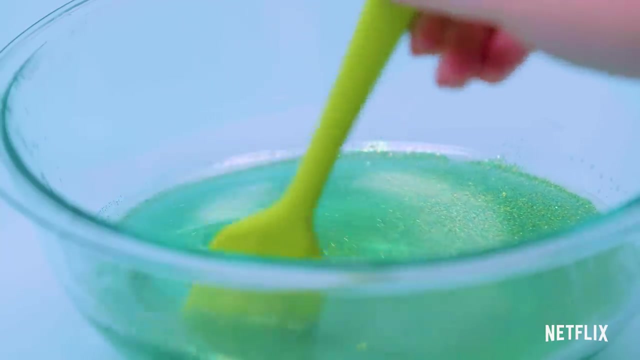